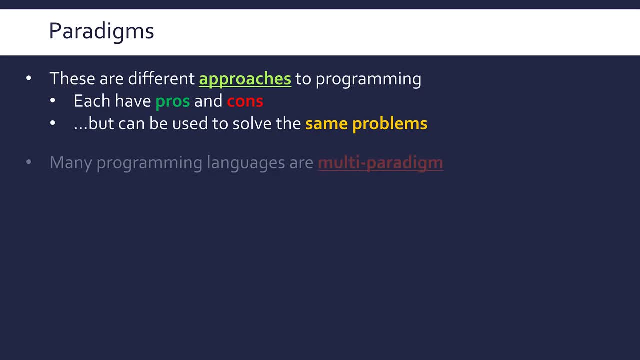 experience with programming in several. so you've got that context, Which is made easier because many- not all, but many- programming languages are said to be multi-paradigm, meaning they support the different approaches, So they might contain constructs which allow you to use multiple paradigms, so, for example, a language like Python. 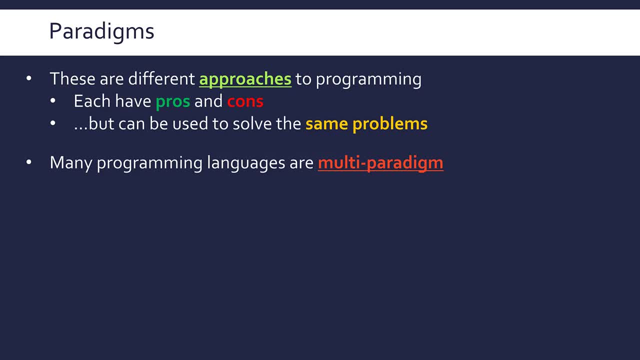 you could completely ignore object-oriented programming and just focus on procedural, but equally it's got object-oriented constructs, and so you can make use of those as well. Having said this, definitely some languages lean towards a particular paradigm. if the creator of that language, or creators of that language, were a particular fan of a particular 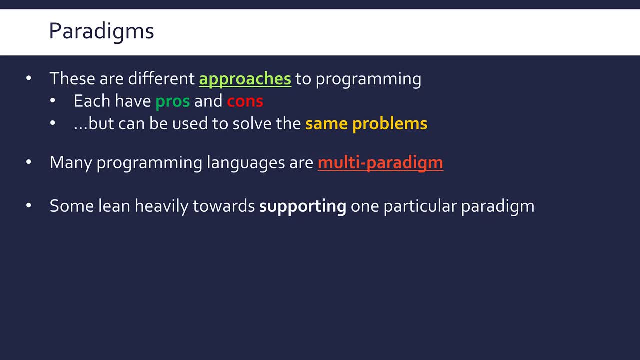 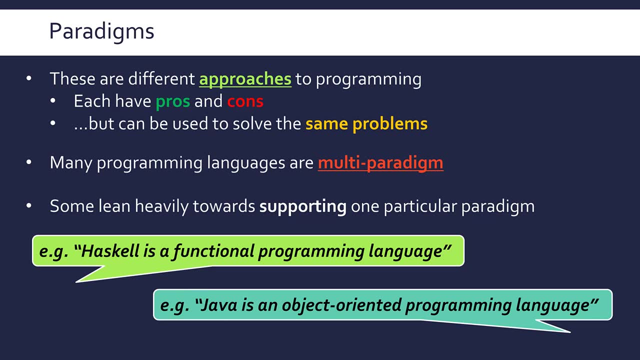 approach. they're going to adapt their language to fit that approach. So, for instance, Haskell is fairly well known as a functional programming language. Java is fairly well known as an object-oriented programming language. those are two paradigms: functional and object-oriented. but it's not always that clear. 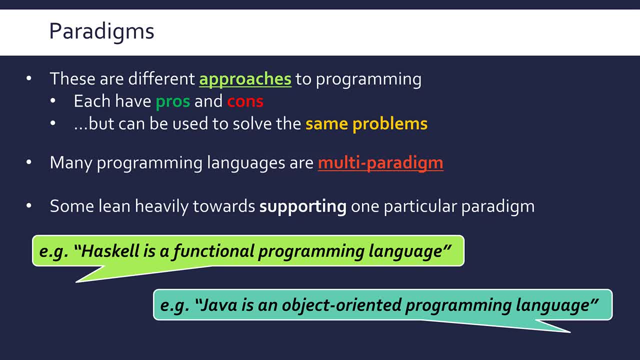 Okay, so not every language you could describe as having one paradigm. even still, a paradigm is often quite loosely defined and it's just a rough approach, a rough set of constructs which, over time, has got labelled under a particular term. You've got to bear in mind programming. 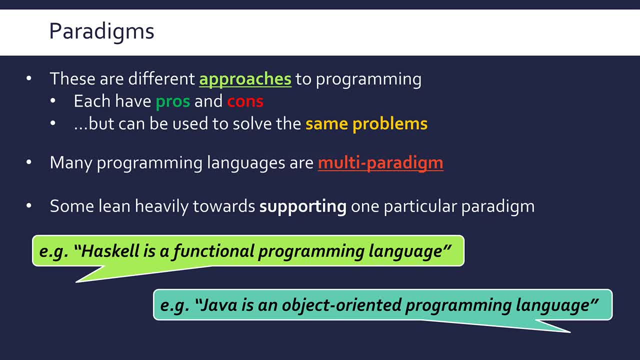 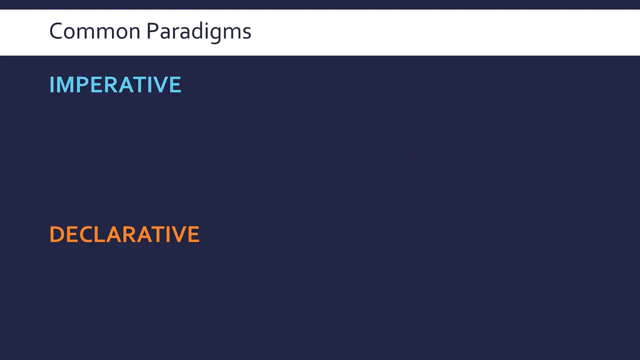 as a field developed very fast from the 1950s onwards, and so things weren't always totally defined, which means 70 years later we've got to sort of try and define stuff ourselves. So let me attempt to do that with some of our big paradigms. Now there are two high 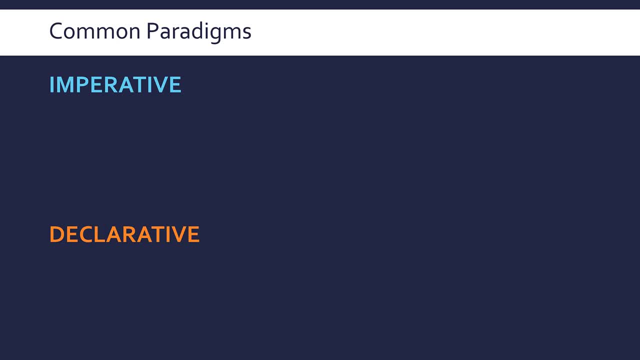 level approaches. as I would personally think of it, We've got imperative languages and we've got declarative languages, and the difference in approaches- imperative languages- have this explicit structure: It's a set of commands. So your program has got commands that specify how to solve your 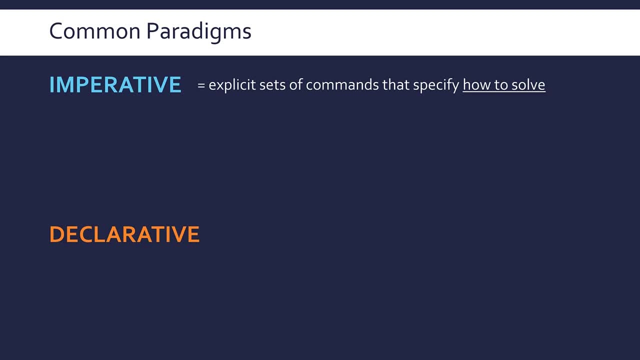 particular problem. You've worked at an algorithm, you've put it into code. it tells you how to solve this problem. so when you follow it, hopefully the problem gets solved, Whereas the approach of declarative languages is not so much telling it how to do it, but instead. 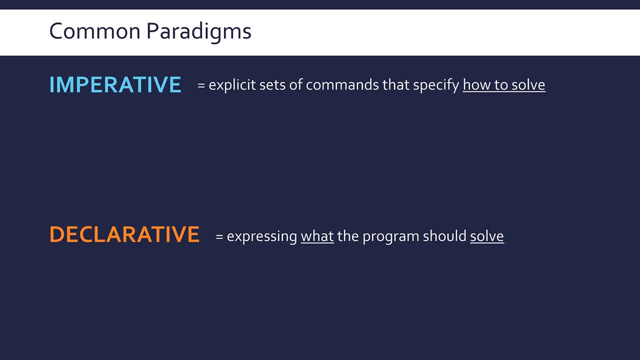 telling it what needs to be done. So you are expressing in your code what the program should solve. So what should the end point be? and you sort of let the compiler or the engine behind the scenes figure out how to get to that point. So imperative, you are telling. 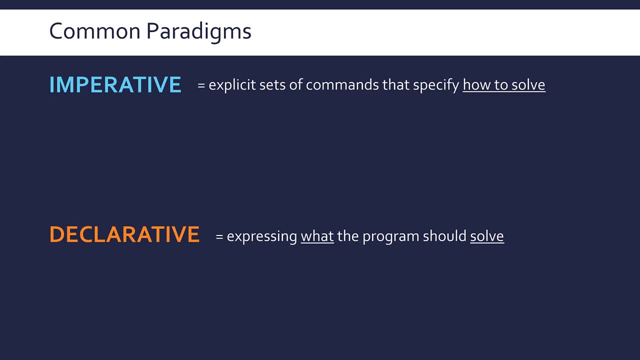 it what to do- declarative- you're telling it where you want to end up with and sort of letting it work on it behind the scenes. Of course, you've got to actually define it very carefully in that point. Now it's not a programming language, but it might give you some context as to what declarative. 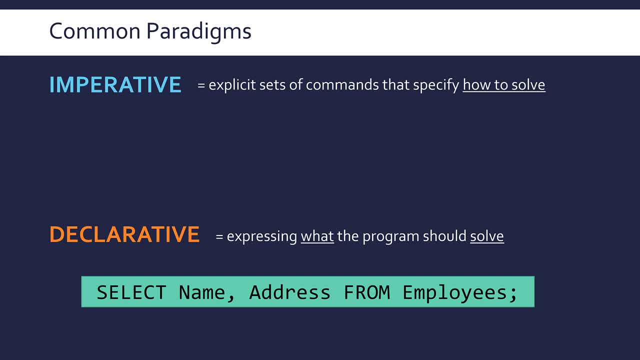 means because quite likely a lot of you watching this will have used a declarative language, even if you didn't necessarily think of it, because SQL for interacting with databases is declarative. So, for example, this tiny bit of SQL code: again, it's not a programming language, but 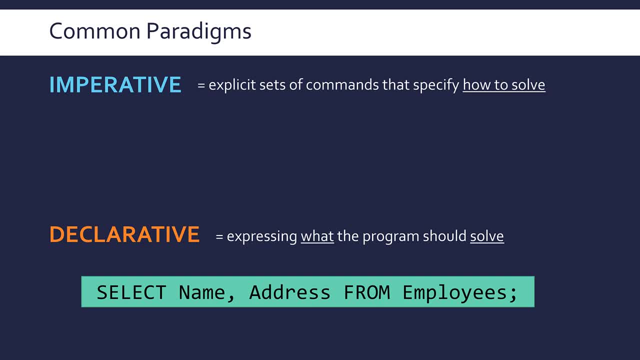 a bit of code: select name and address from employees. you're telling it what you want. you want the name and address column in the employees table, but you're not telling it how to get it. you're just saying what you want in the end and the database system will. 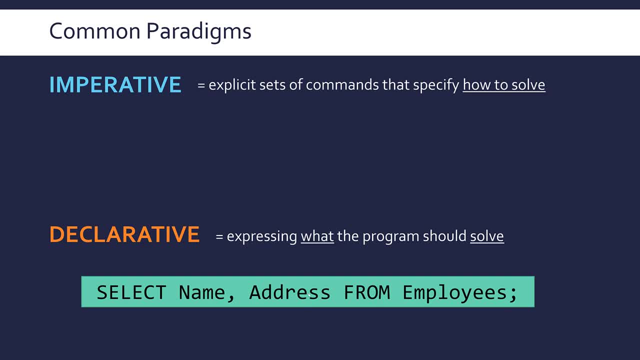 figure out how to get this for you. you're not really worried about how exactly it's doing it. Now, within imperative we've got a few other paradigms as are generally defined, and the big one inside declarative for actual programming is the functional paradigm. 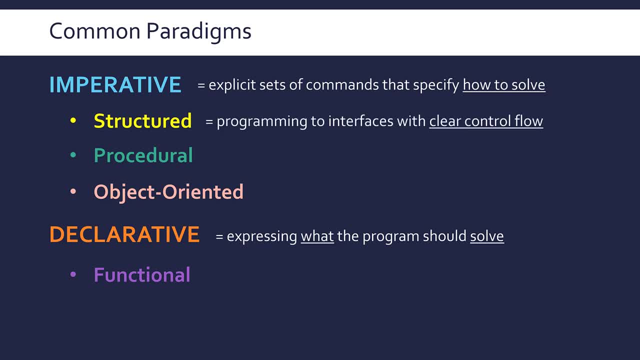 So structure programming is often considered a part of procedural, but for now let me just separate it because they are a tiny bit different. Structure programming is really trying to be ultra clear, ultra organized in your code. So you're programming to subroutine interfaces, you're trying to abstract as much as possible. 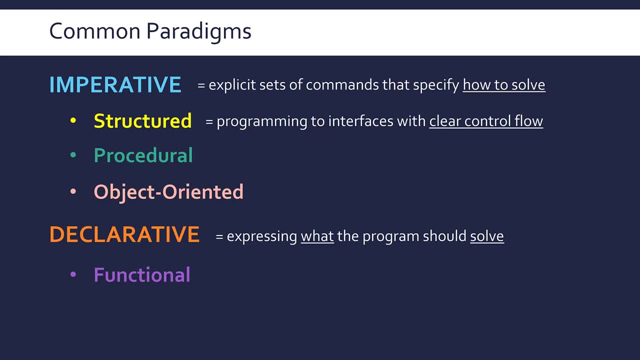 and use parameters, use return values and within your code you've got clear control flow. You've got selection iteration where you can, so that the logic inside your program is really, really clear. Now this is often part of procedural, because really you're using subroutines and the procedural 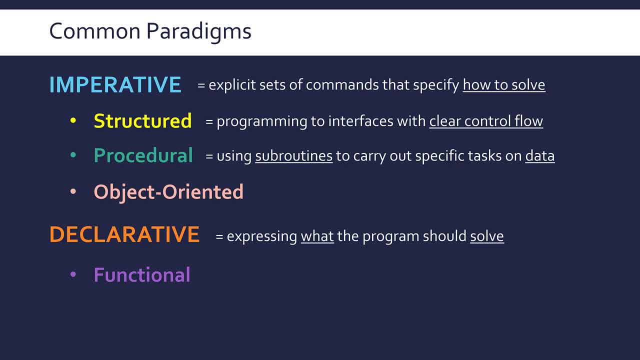 paradigm is all about using these subroutines to carry out specific tasks on data. So you've got many subroutines, which are blocks of code which perform one job. Now you could produce some structured code without using any subroutines, but in reality, 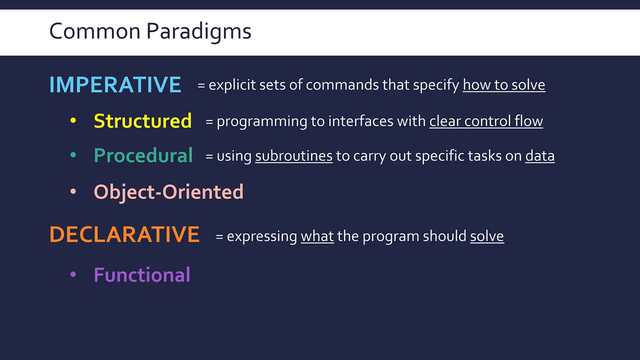 if you're doing procedural programming, You should be aiming to do structured programming as well. Object-oriented programming has its own constructs. We've got objects and classes, and one of these constructs- objects- are trying to encapsulate both behavior and data. So, whereas procedural, we've got data being worked on by subroutines, but they're kind.